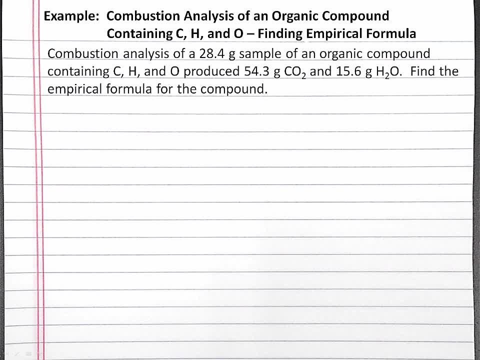 In this example problem we'll find the empirical formula of an organic compound containing carbon hydrogen and oxygen using combustion analysis. Our problem reads: combustion analysis of a 28.4 gram sample of an organic compound containing carbon hydrogen and oxygen produced 54.3 grams CO2 and 15.6 grams H2O. 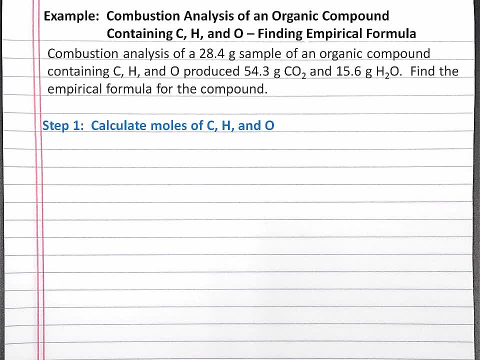 Find the empirical formula for the compound, Our first step will be to calculate the moles of carbon, hydrogen and oxygen. In this problem. we assume that all of the carbon in our organic compound is incorporated into the 54.3 grams of carbon dioxide, so we begin our dimensional analysis with 54.3. 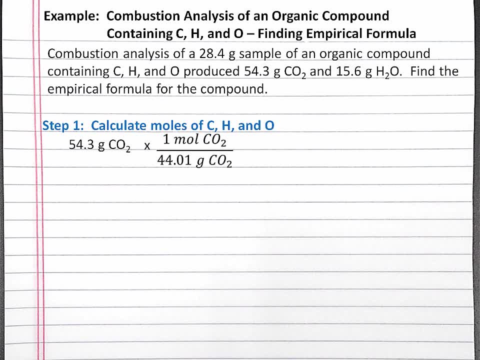 grams of carbon dioxide and we convert into moles of carbon dioxide using the molar method. We convert into moles of H2O using its molar mass and then into moles of carbon using the ratio from the chemical formula and we'll get 1.23 moles of carbon. 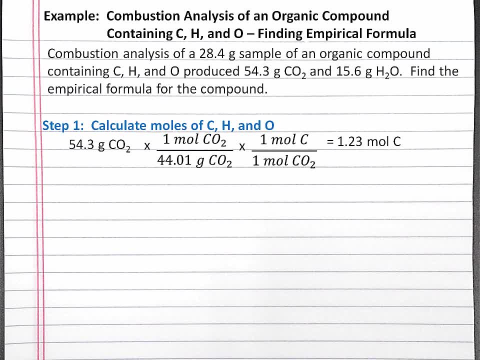 We also make the assumption that all of the hydrogen in the organic compound gets incorporated into the H2O. So, beginning with 15.6 grams of H2O, we can convert into moles of H2O using its molar mass and into moles of hydrogen using its molar method. 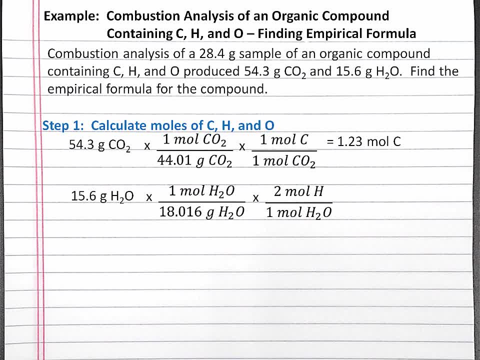 In this example we use the ratio from the chemical formula and we'll get 1.73 moles of hydrogen in our sample. To calculate the moles of oxygen in our sample, we first have to determine the mass of oxygen. We know that the total mass of our sample is composed of the mass of carbon and the 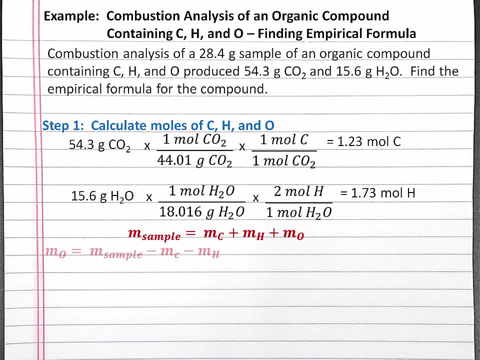 mass of hydrogen and the mass of oxygen. so we can solve for the mass of oxygen by taking the mass of the sample Subtract the mass of carbon and the mass of hydrogen. We're given the mass of the sample in the problem is 28.4 grams. 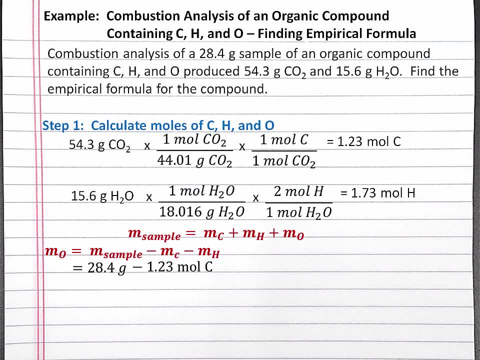 And we calculated that we have 1.23 moles of carbon and we can convert this moles of carbon in our sample into grams of carbon using its molar mass. And we also calculated that we have 1.73 moles of hydrogen in our sample and we convert.